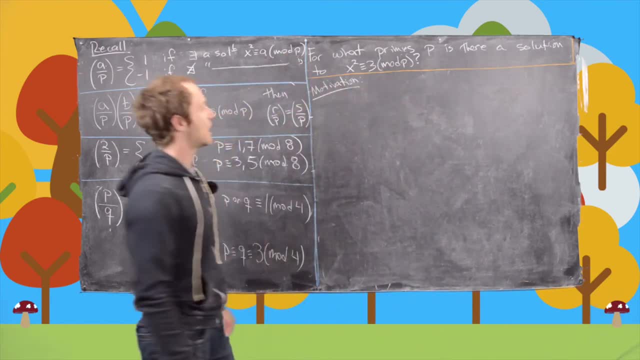 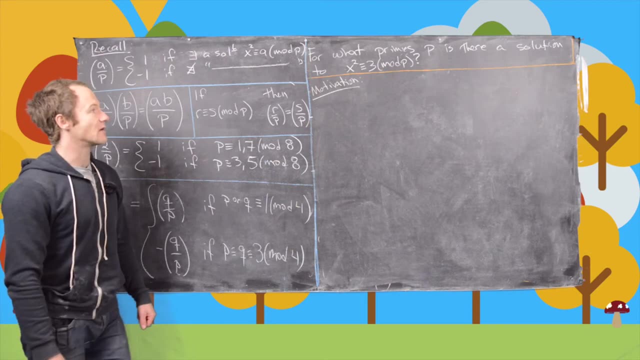 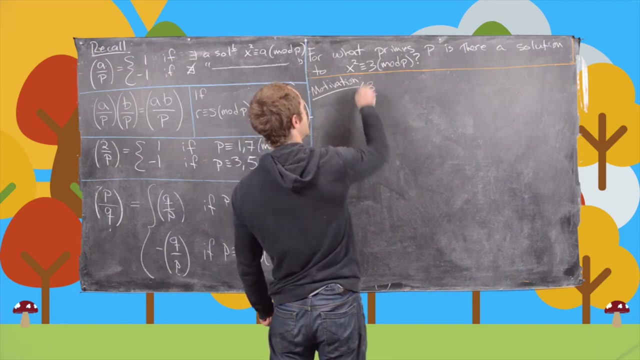 there's no minus sign otherwise, Okay, good, So now we're going to use the Legendre symbol and all of these properties, including quadratic reciprocity, to answer this question, And so now our motivation will be the following: So what we want to determine is: when is 3 by p equal to 1.. So that's the. that's the real question. 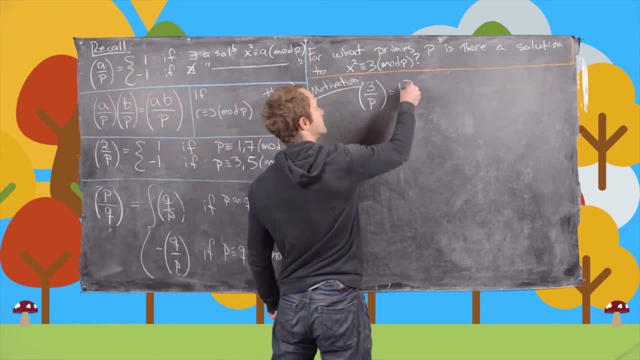 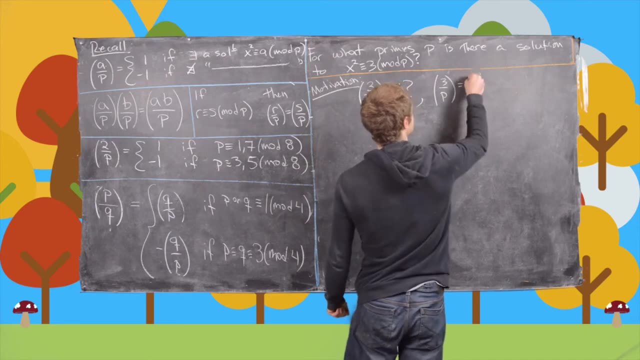 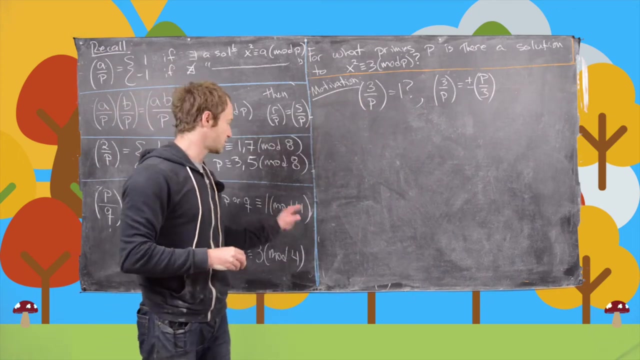 is when is 3 by p equal to 1.. Good, And then we'll also notice that 3 by p equals plus minus p by 3.. Okay, good, And now notice that this plus minus depends on the congruence mod 4 of p. and then 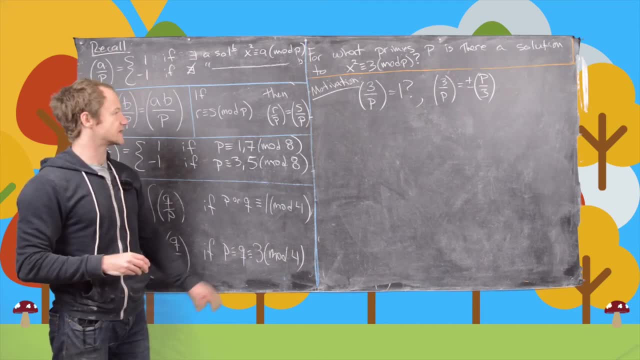 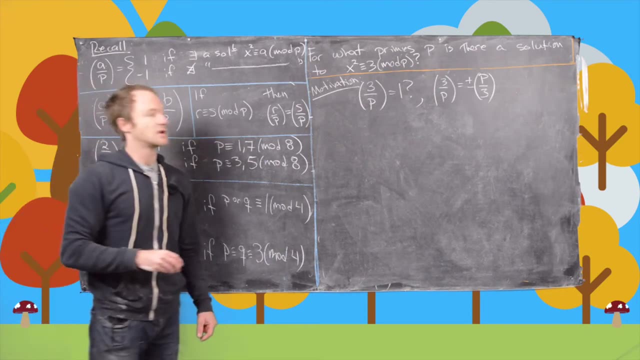 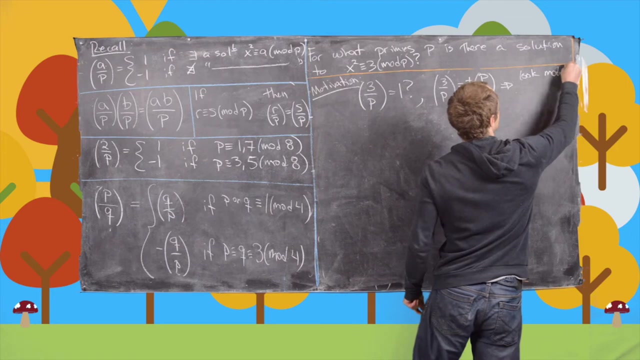 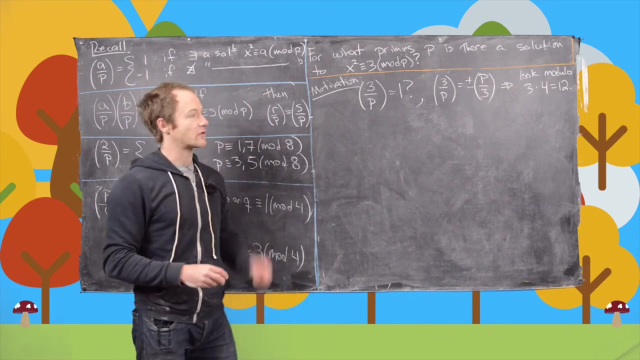 a simple reduction of the Legendre symbol itself will depend on the congruence of p, mod 3.. Good, So that tells us that maybe we should look Modulo 3 times 4, which is 12.. Okay, So again let's reiterate why we want to look modulo 12.. 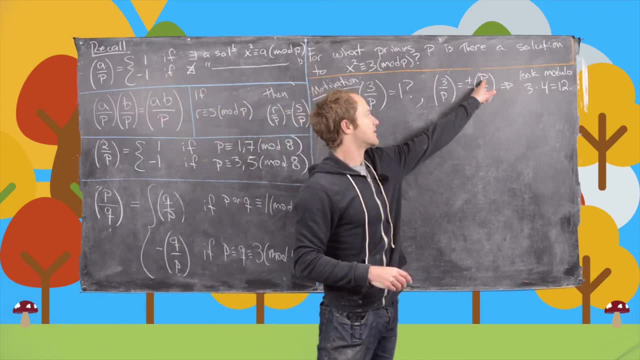 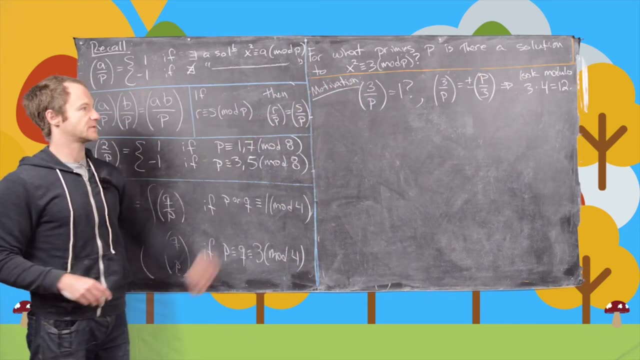 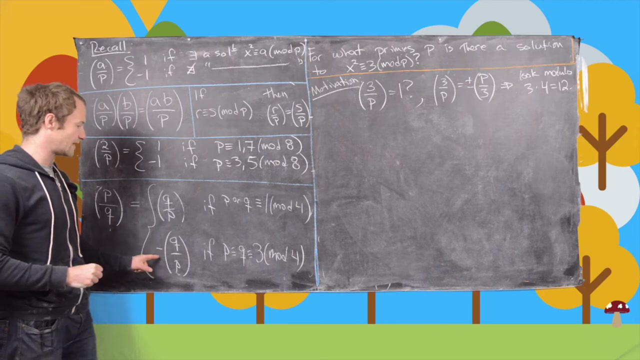 So we want to look. modulo 3 because considering p. mod 3 will allow us to simplify this Legendre symbol using this property. Good. And then working. mod 4 will allow us to decide. if that flip came with no minus sign, curve Right. 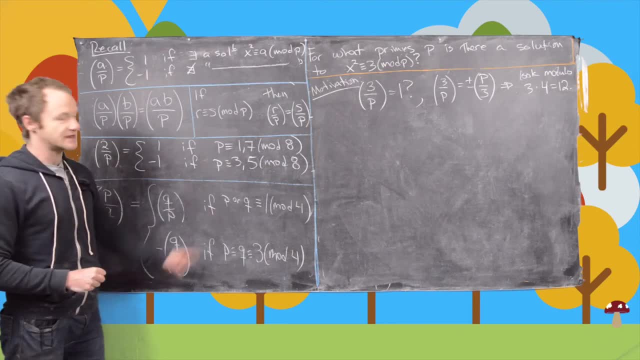 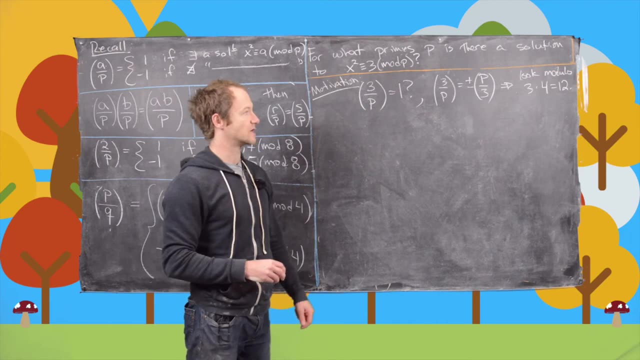 Or Right, Or Right, Right, Right Or a sign using this quadratic reciprocity property. Okay, good. So, all in all, we have to work modulo 3 times 4, which is 12.. Okay, so that's going to break down into four cases. So case: 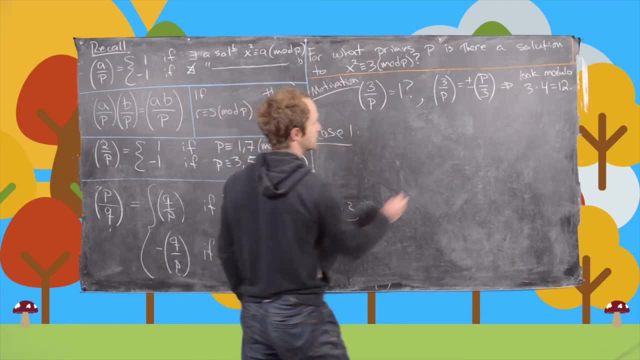 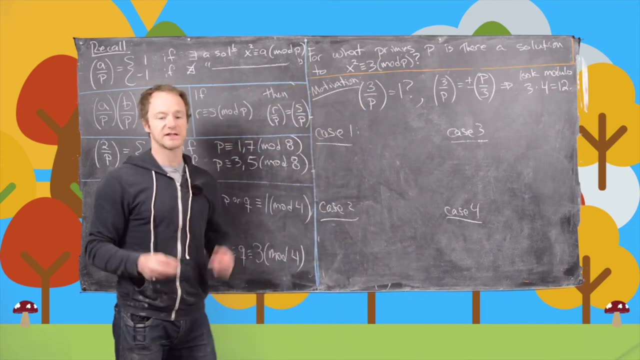 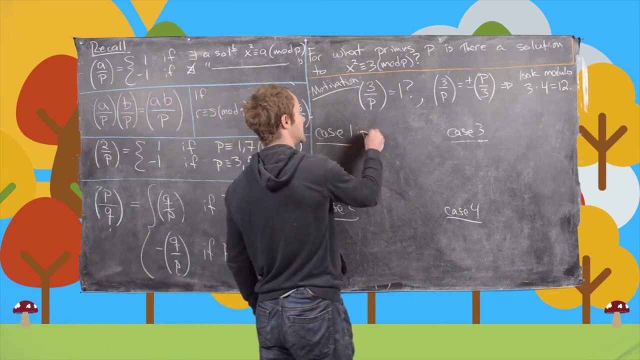 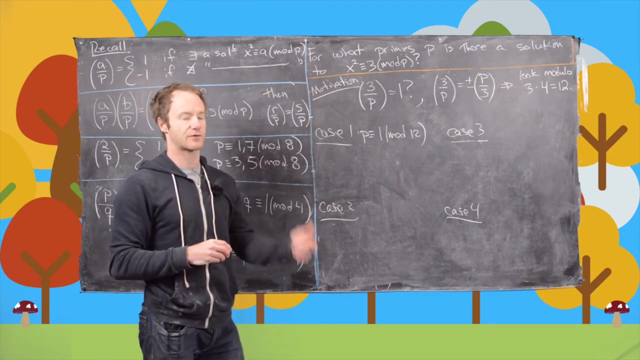 number one, case two, case three and case four, And those cases will be all possible primes and their congruence class mod 12.. So obviously you could have p is congruent to 1 mod 12.. That's a type of prime mod 12.. Notice you can't have 2 mod 12, 3 mod 12,. 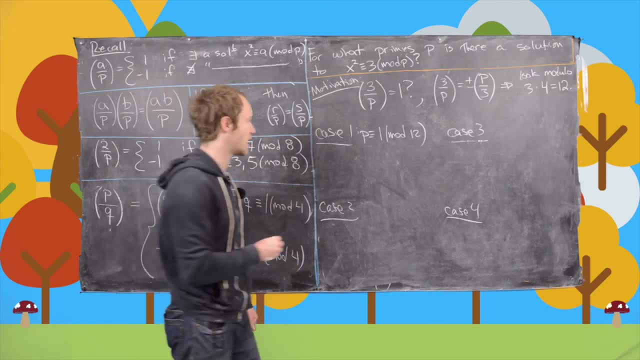 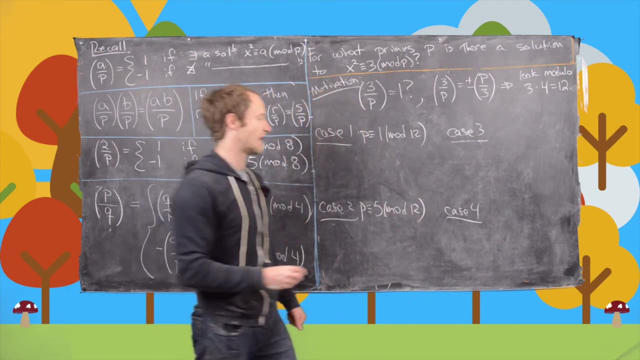 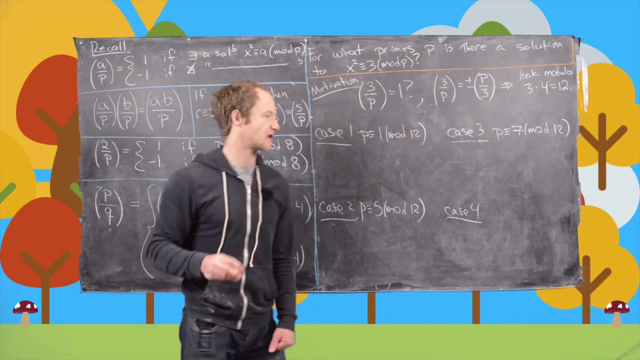 or 4 mod 12,, because those are not relatively prime to 12.. You can have p is congruent to 5 mod 12.. Again, you can have p is congruent to 7 mod 12.. You can't have 6 mod 12, because those are not relatively prime. You can't have 8,, 9,. 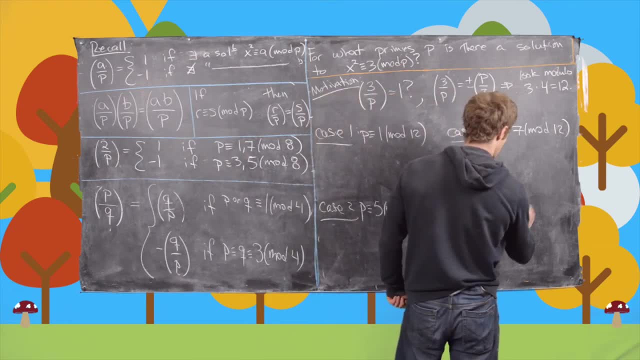 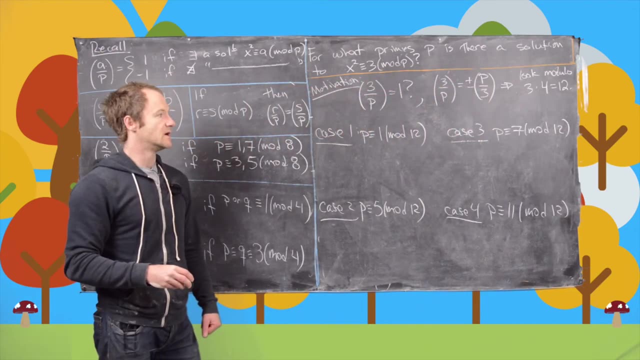 or 10 mod 12. And then you can have p is congruent to 11 mod 12.. You obviously can't have p is congruent to 0 mod 12, because then it would be divisible by 12 itself. Okay, and so now. 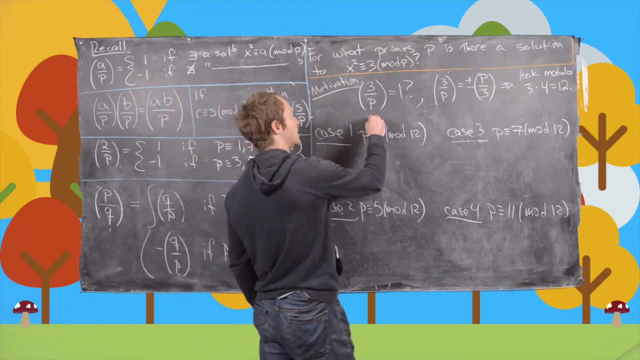 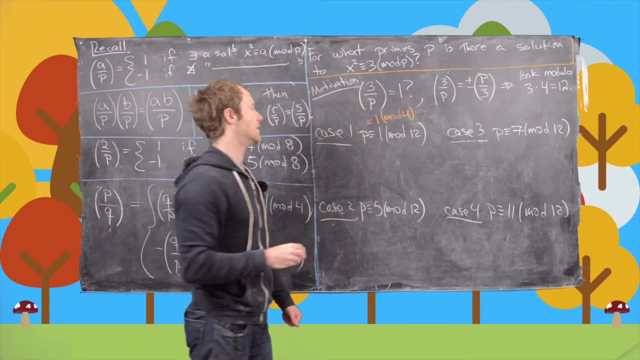 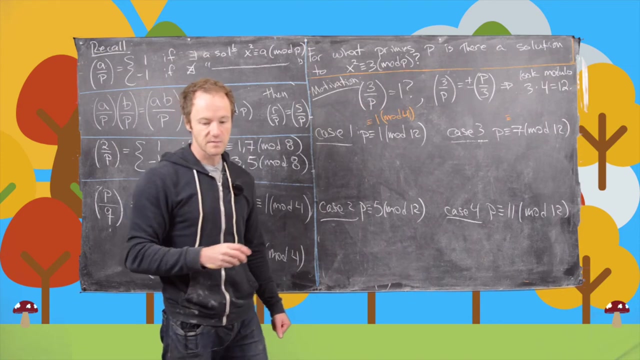 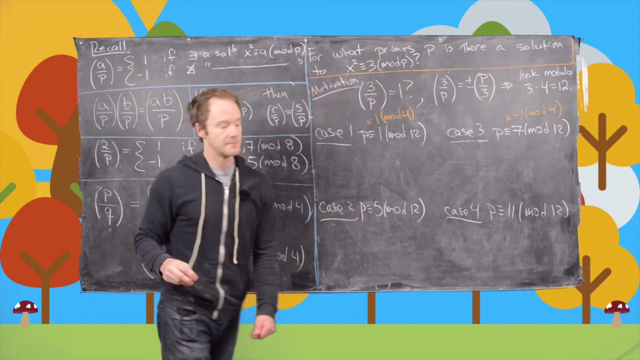 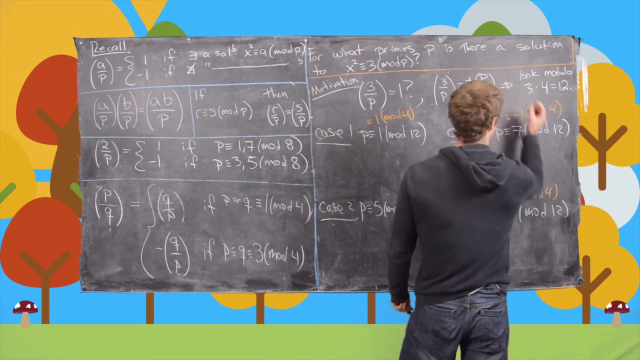 let's also notice that if it's 1 mod 12, it's also congruent to 1 mod 4.. Good, And if it's 7 mod 12, it's congruent to negative 1 mod 4. Okay, good. If it's 11 mod 12, it's congruent to negative 1 mod 4.. And I guess I should say: 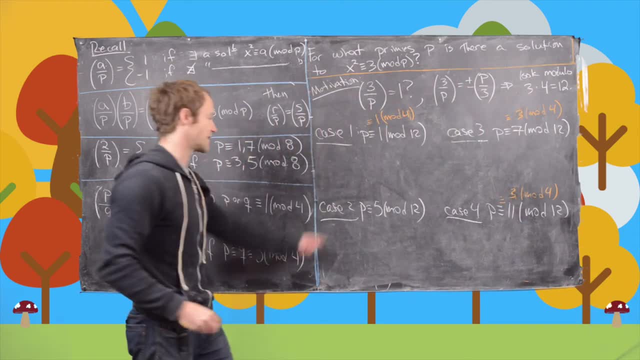 this is 3 mod 4, to be in line with our formula over here. If it's 5 mod 12, it's clearly congruent to 1 mod 4.. So if it's 7 mod 12, it's congruent to negative 1 mod 4.. 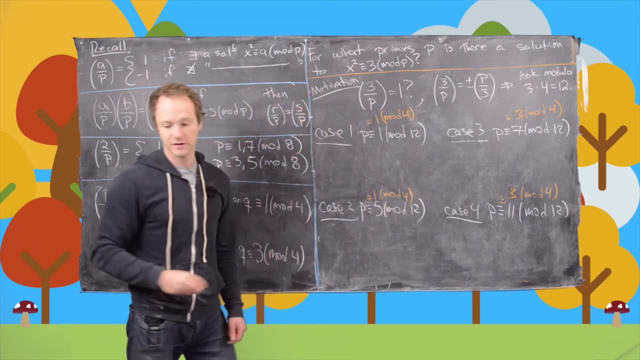 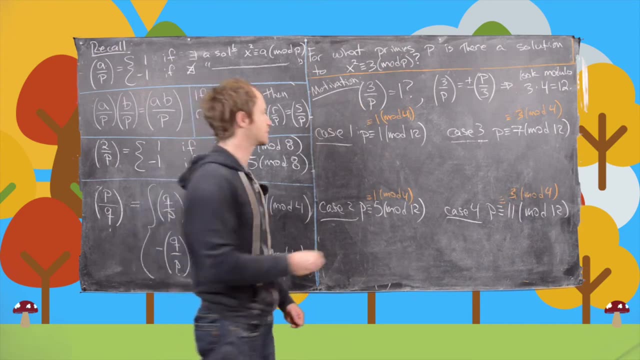 It's congruent to 1 mod 4. Good. So those are those simplifications. And then let's also notice that if it's congruent to 1 mod 12, it's also congruent to 1 mod 3.. Good, If it's congruent. 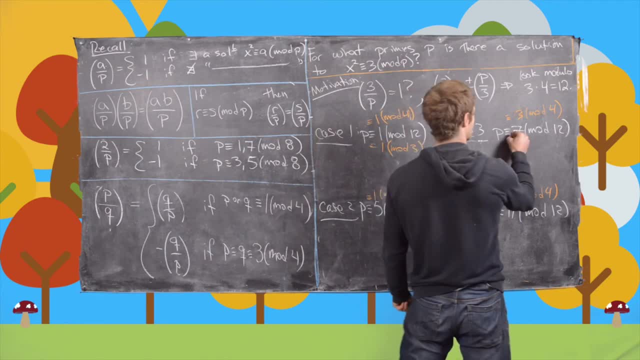 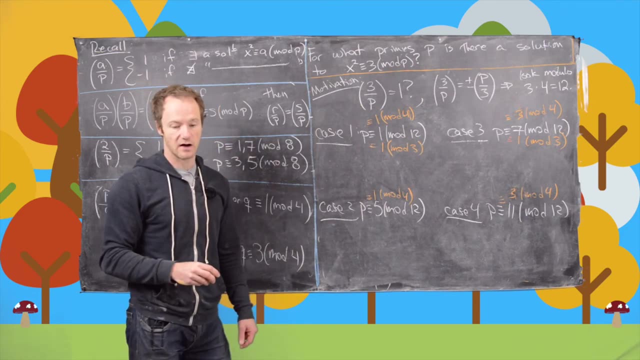 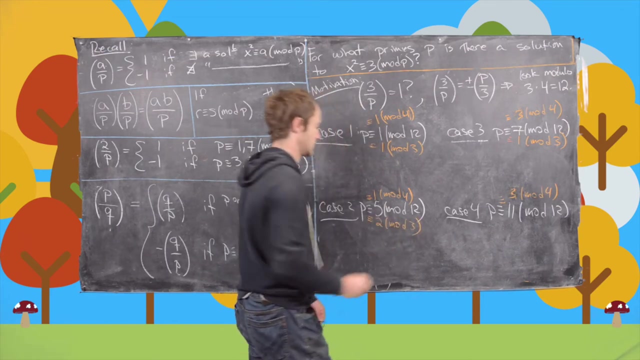 to 7- mod 12,, it's congruent to 1 mod 3. Good. If it's congruent to 5- mod 12,, it is congruent to 2 mod 3. Good. And then, if it's congruent to 11- mod 12, it's also congruent to 2 mod. 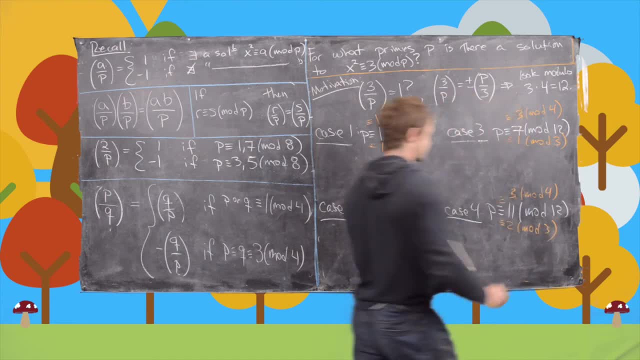 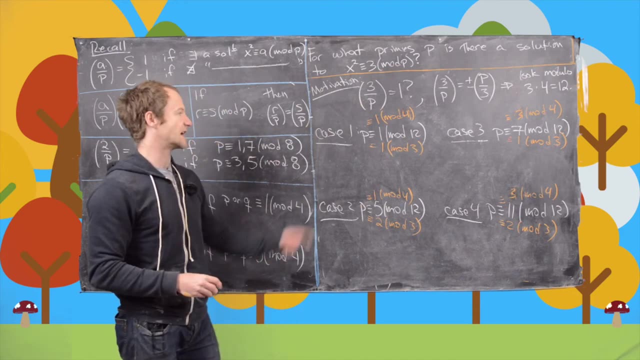 3. Good, So all that orange stuff is like seen as kind of scratch work, but that's going to be used to help us as we work through this. Okay, so let's see We have 3 by p. So this: 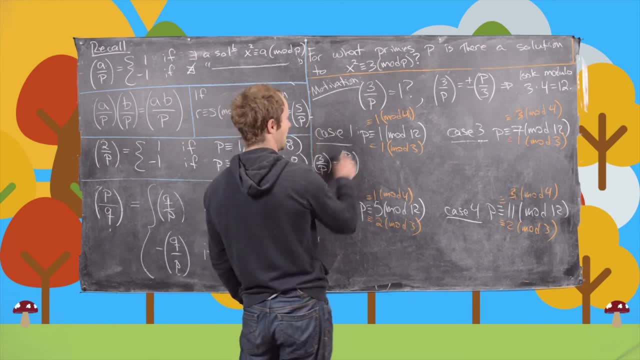 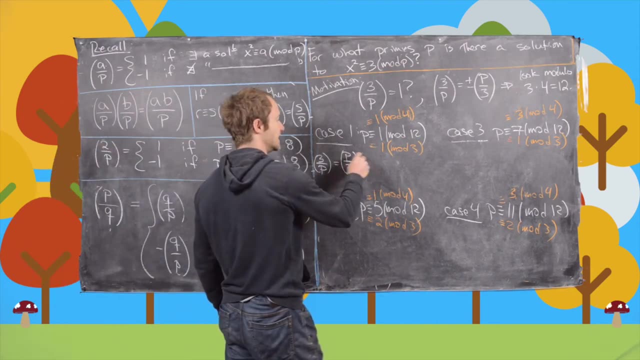 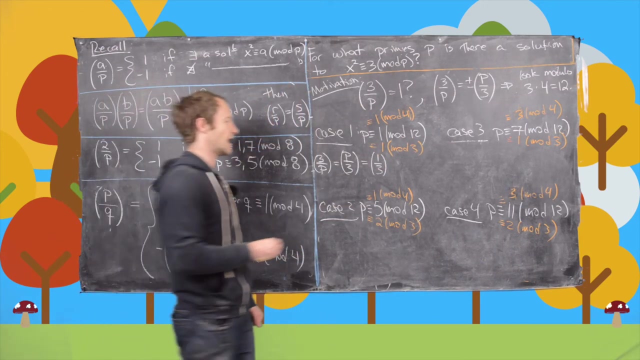 is equal to p by 3.. We can do that because we have 1 mod 4 here as p. Good, And now the next thing that we can do is reduce this to 1 by 3, because p is congruent to 1 mod 3.. Great, And then we 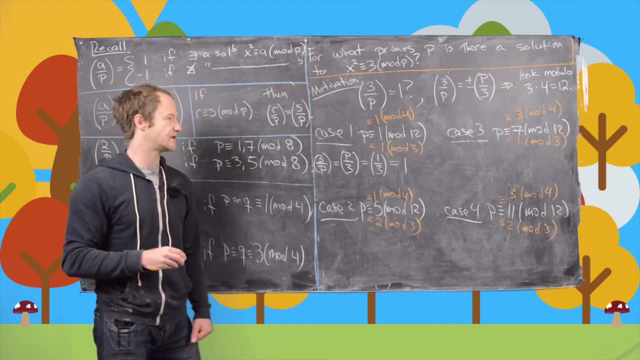 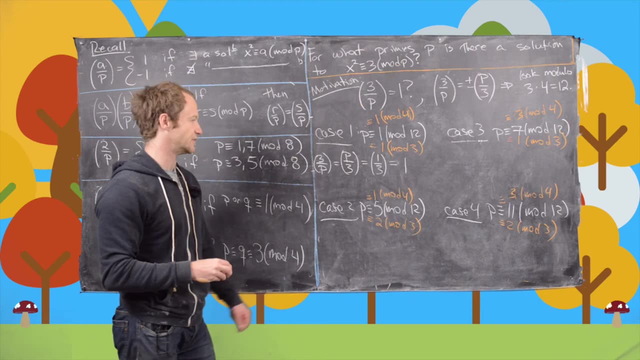 know that the answer to this is 1, because 1 squared is equal to 1.. It's obvious that 1 is the quadratic residue. Okay, so we're done with that. Now let's move on to case number 2.. Okay, so now we'll do 3 by p. So this is going. 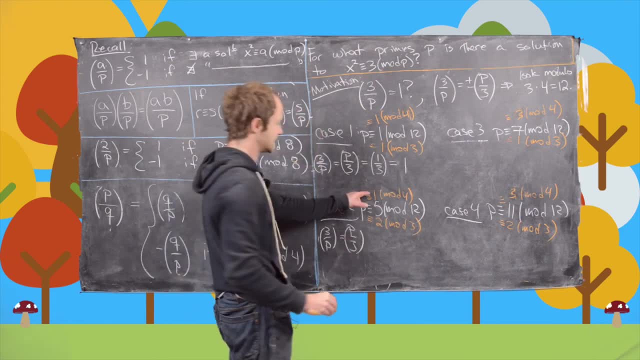 to be 1 by 3.. And then we're going to do 3 by p, And then we're going to do 3 by p. So this is going to be equal to p by 3, again because we're using the property that p is. 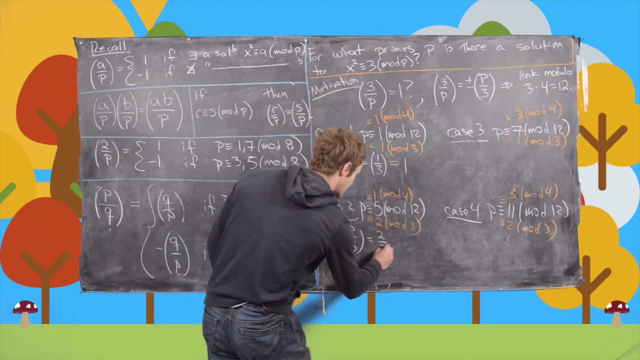 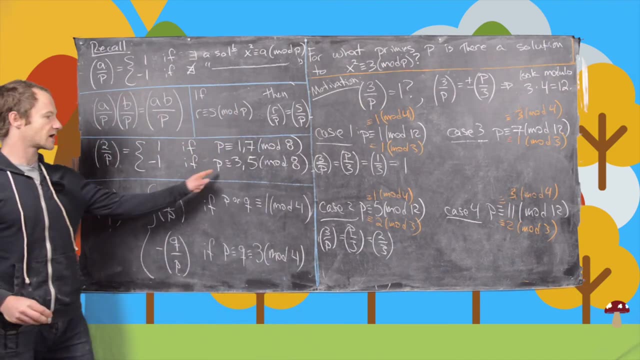 1 mod 4.. But now this is 2 by 3.. Okay, great. Now we go over here and look at this property: When is 2 a quadratic residue? And look, now we have p, which is the denominator. now It's. 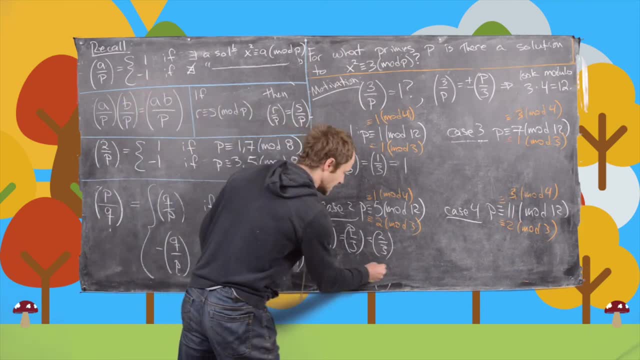 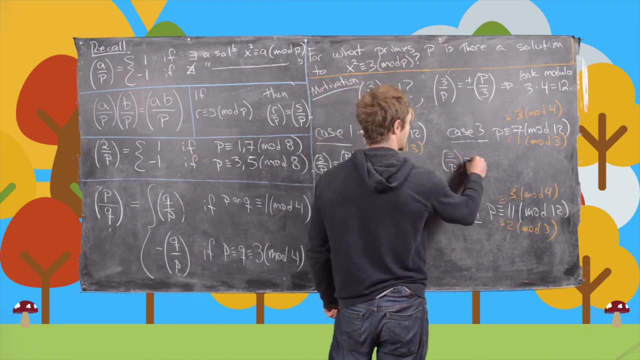 3, is equal to 3.. So the answer to this is negative, 1.. Okay, so now let's move on to the next one. So we have 3 by p, So now we can flip that to p by 3.. But we need to include a minus sign, because p and 3 are both congruent. 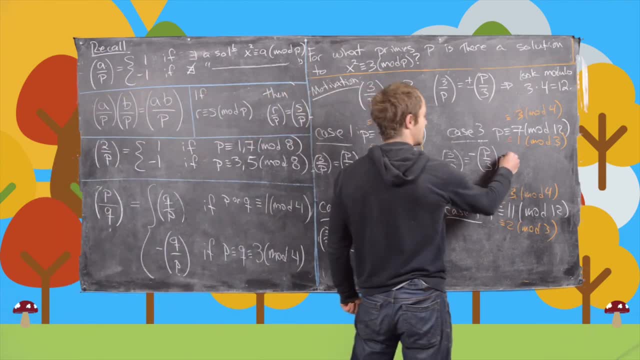 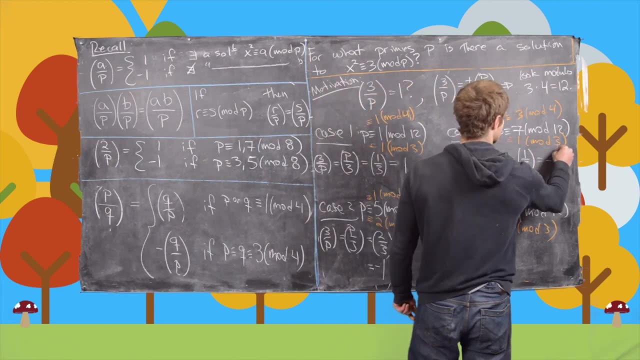 to 3 mod 4. Great, And now we can reduce this modulo 3.. So that gives us minus 1, 1 by 3.. But that's obviously going to be minus 1.. So the minus sign comes from here, And then 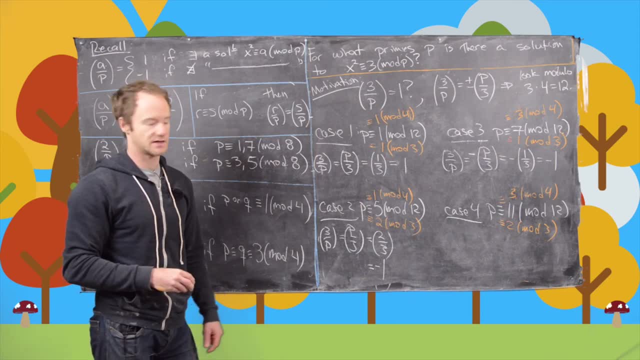 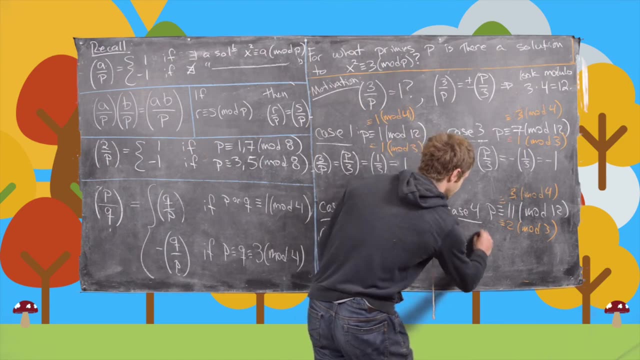 1 by 3 is obviously 1.. So you get minus 1 in the end. Okay, good. So now let's look at this last one. So we have 3 by p, So we can flip that to p by 3.. But we have to pick up a minus sign, because they're both. 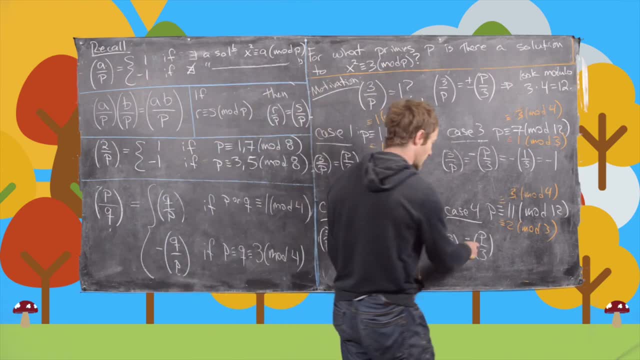 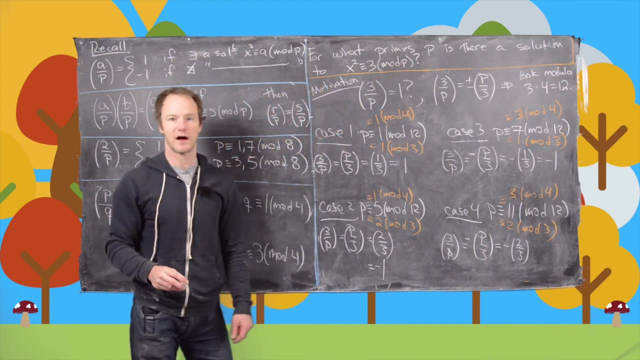 congruent to 3, mod 4.. Okay, good, And now we can replace p with 2. So we have negative 2 by 3.. Again, because p is congruent to 2 mod 3.. And then, finally, we know: 2 by 3 is. 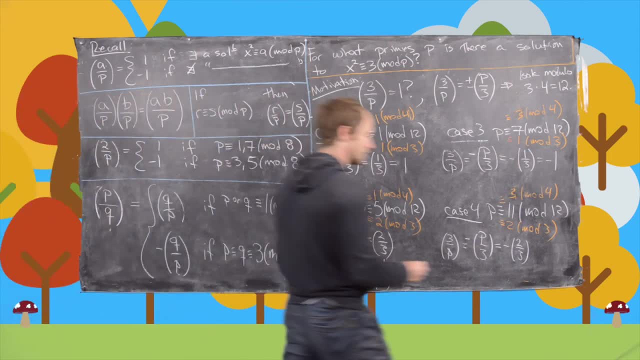 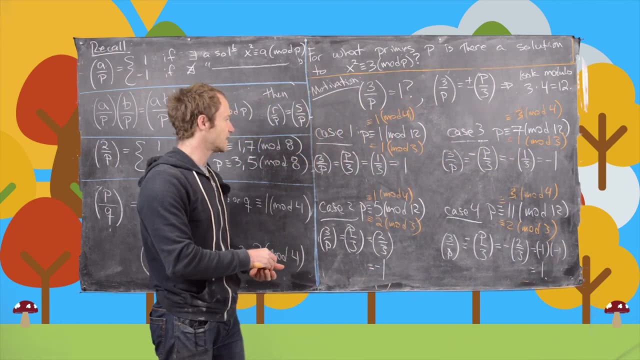 equal to negative 1 by this property which we used before. So this is equal to negative 1 times negative 1, which is 1.. We look at this in total. Notice that here we get a 1.. Here we get a 1.. So the answer: 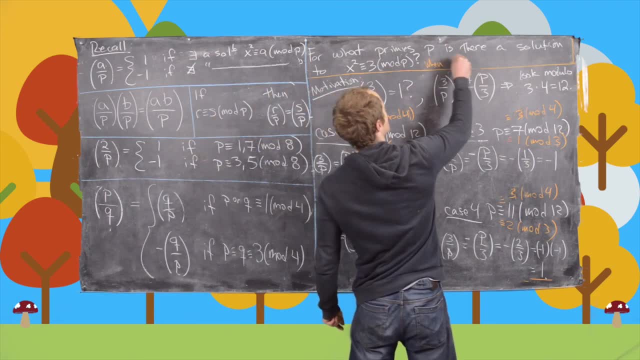 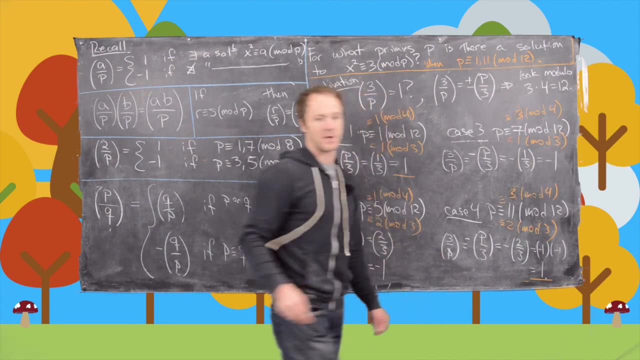 to this is when p is congruent to 1 or 11 modulo 12.. Okay, good, And that's the end of the video. 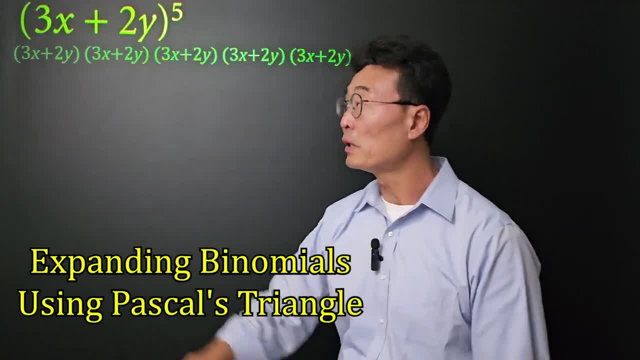 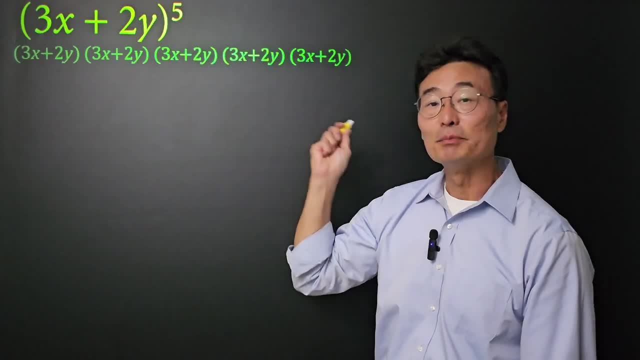 In order to take the binomial 3x plus 2y to the fifth power, you have to multiply 3x plus 2y five times. This could be quite a bit of work. Here's a better way. Let me introduce you to. 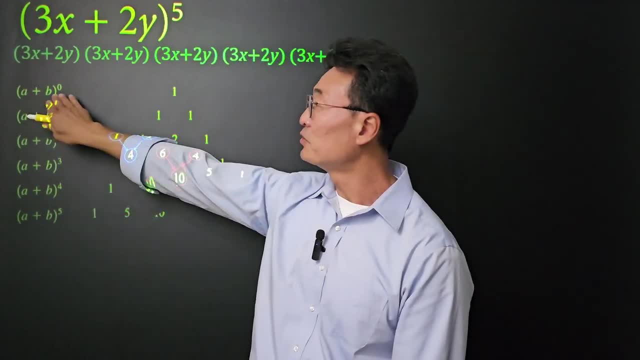 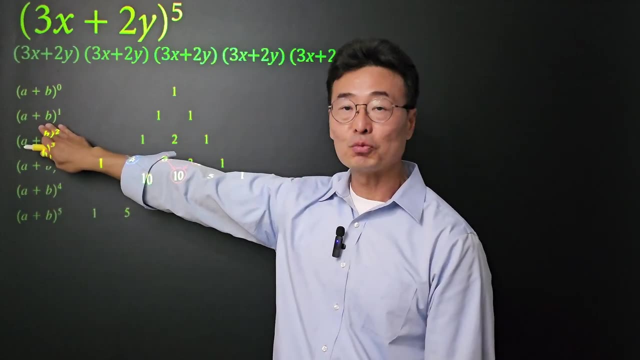 Pascal's triangle. When you have a plus b to the zero power, of course it's going to be one, because anything to the zero power is always one. And then, when we have a plus one to the first power, because the coefficient of a is one and coefficient of b is one, we have one and one. 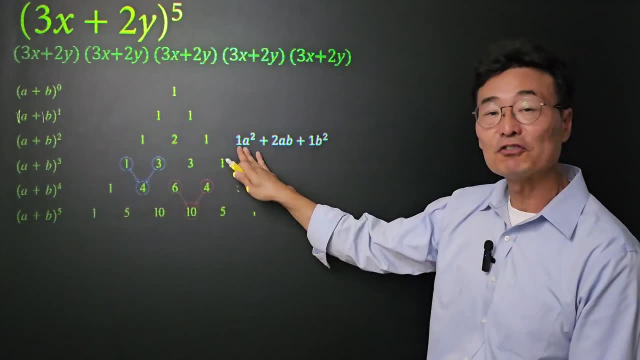 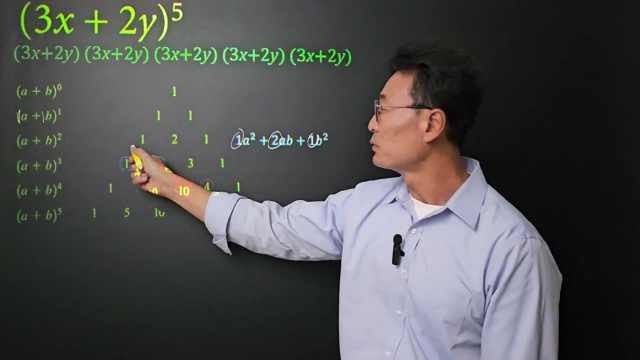 And then when you do a plus b squared, we get one a squared plus two ab plus one b squared. So from the one, two and the one, that's where we get the one, two and the one in the Pascal's triangle.